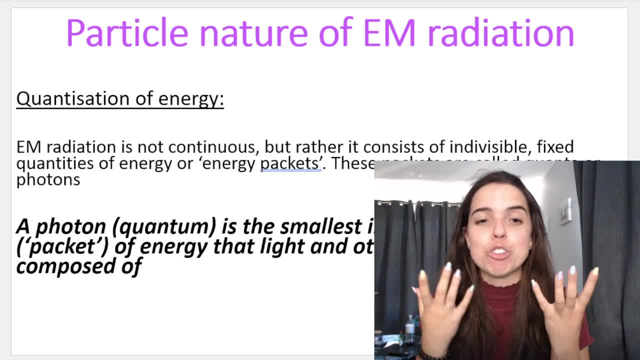 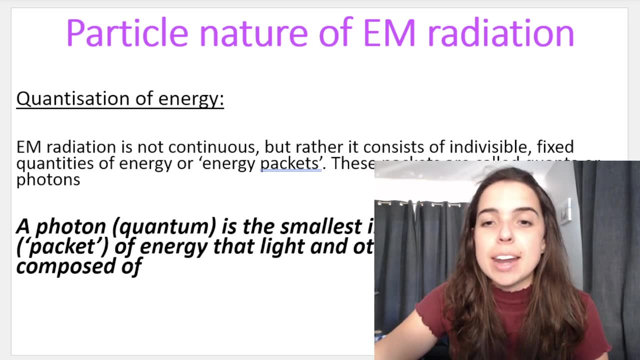 this. Well, we need to look at it in terms of light or electromagnetic radiation. So electromagnetic radiation is not actually continuous. I want you to think of it as having little, tiny energy packets or pockets. So it says here behind me that electromagnetic radiation is not continuous. 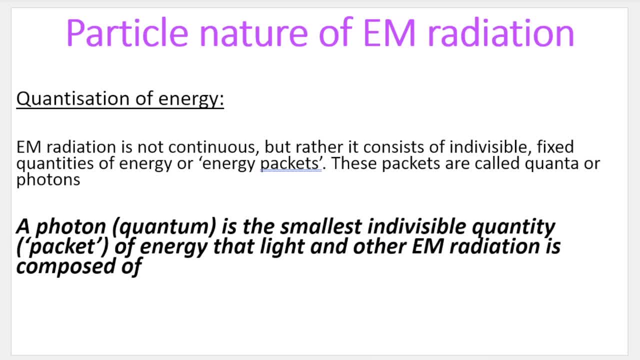 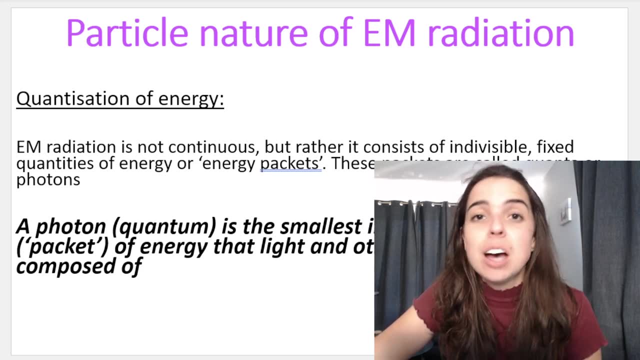 but rather it consists of indivisible- which means you can't divide it- fixed quantities of energy or packets of energy, and we call these quanta or photons, So we mostly refer to it as photons. so from this point out I will be referring to it as photons. So a photon or quantum is the 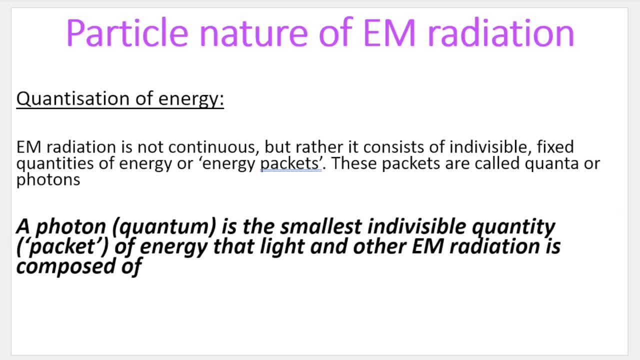 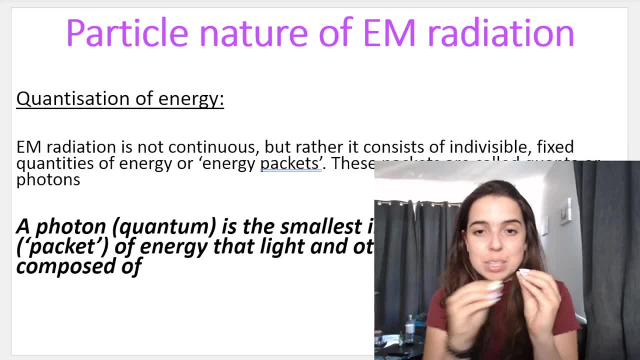 smallest indivisible quantity. It's a packet of energy that light and other electromagnetic radiation is composed of. So it's a packet of energy that lights and other electromagnetic radiation is composed of. So it's the smallest indivisible little packets of energy that light is composed of. So if I shine, 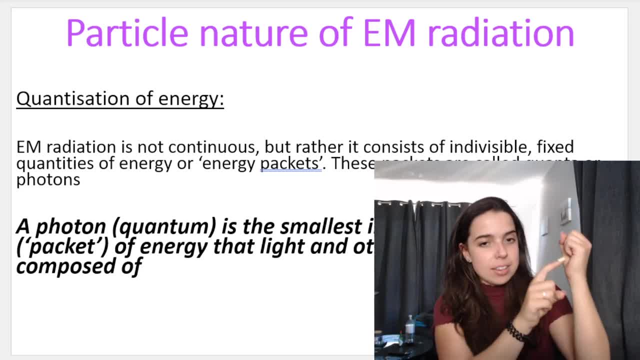 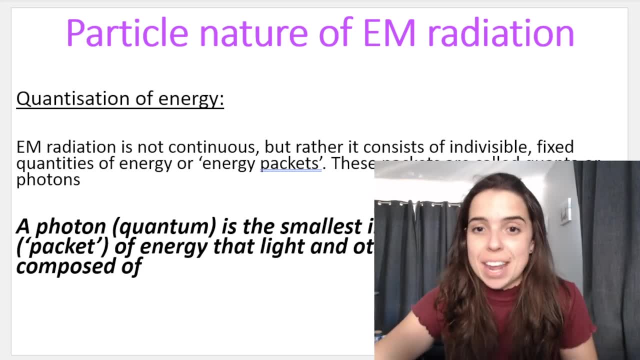 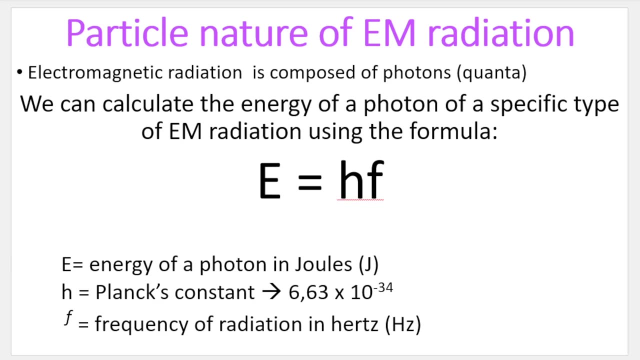 a beam of light- and you can see that light beam- that is actually composed of thousands, millions of photons. Those are little packets of energy that are contained in light And we can calculate the energy of those photons using a very, very particular formula. So that's the formula there. 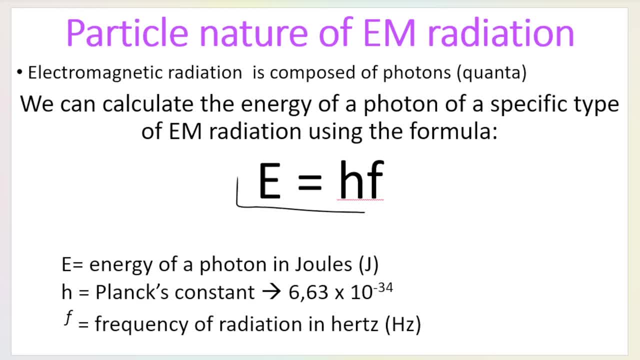 on the screen. You get this on your data sheet or your formula sheet, so it's given to you in a few exams. E is the energy of the photon and it's measured in joules or J. So the unit for energy is joules or J H. this is a constant, Planck's constant, And this number over here 6,63 times. 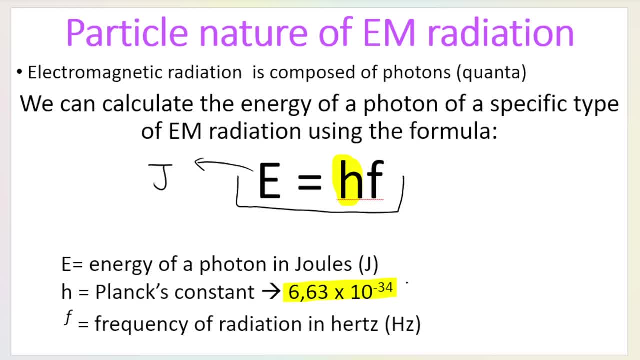 10 to the negative 4,. because it's constant, it means it'll never change. So it'll always be that number And this number you can find on your data sheet or on your formula sheet. Okay, it'll be written there for you. And F is the frequency of the radiation, or. 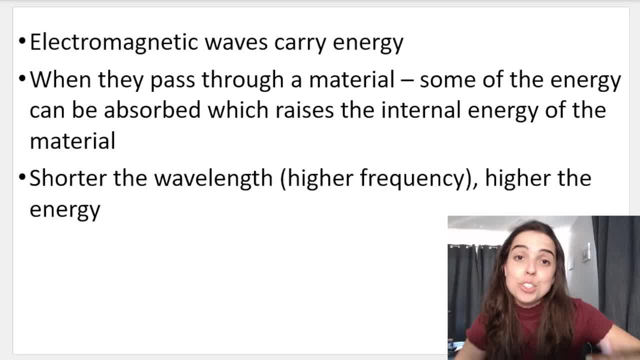 frequency of the light measured in Hertz. So remember, electromagnetic waves carry energy. They carry these photons, these packets of energy. So when we have the electromagnetic waves, so think about maybe an X-ray or infrared light or UV light- they pass through the material. 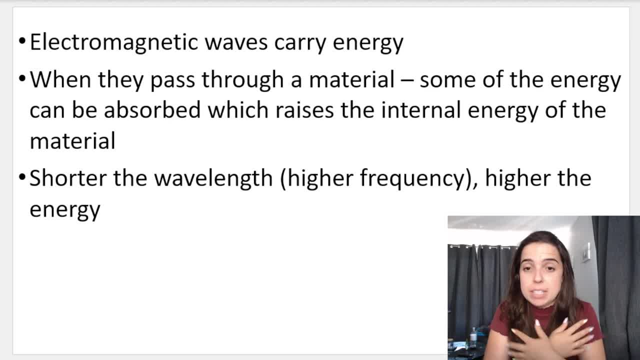 And some of that energy can be absorbed by that material, which raises the internal energy of the material, which is why some materials heat up. for example- And just remember what we discussed in the other video- The shorter the wavelength, the higher or the bigger the frequency, And if you have a bigger 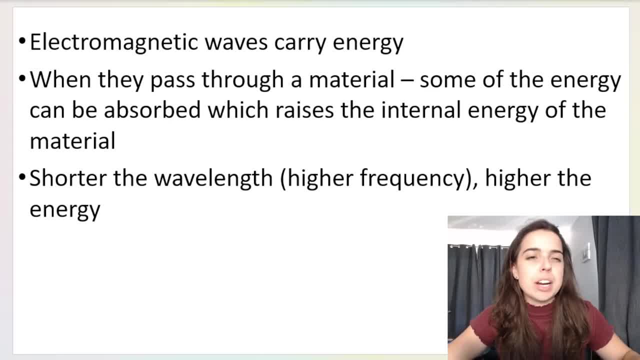 frequency, you have a bigger energy. So remember that formula that I just showed you: E energy is equal to HF. What that means is that if frequency gets bigger, E gets bigger. What relationship is that called? again, That's called directly proportional. That symbol is used for. 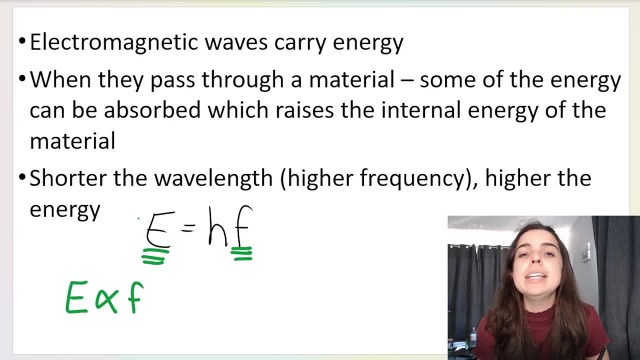 directly proportional. It means that if F doubles, E doubles. If F gets three times bigger, E gets three times bigger. That's what a direct proportion relationship is. If F halves, E will half, So they increase or decrease by the same proportion. They. 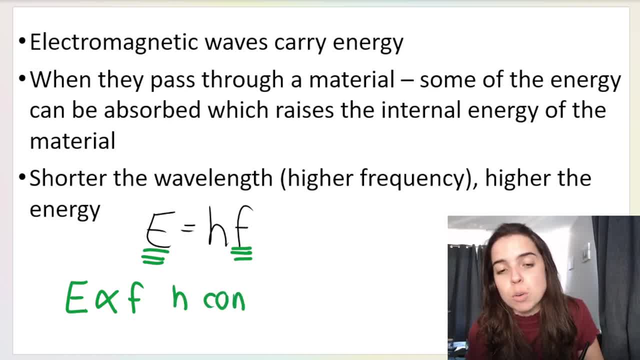 match one another in that way. But H must be a constant in order for this relationship to be true, which it is. H is Planck's constant. It's always the same value. So we know, the higher the frequency of the wave, the higher the energy, And if you watch the previous video, you will know that gamma. 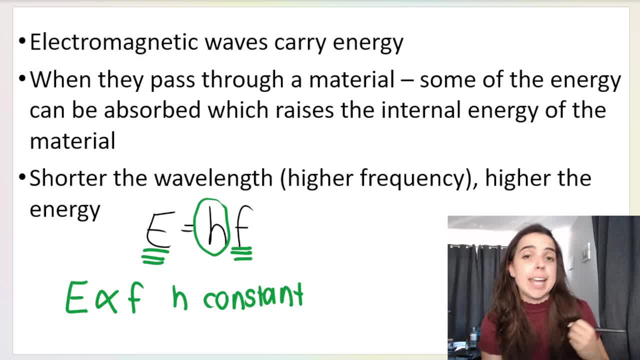 rays have the highest frequency. So if you watch the previous video, you will know that gamma rays have the highest frequency. So if you watch the previous video, you will know that gamma rays have the highest frequency, which means they have the highest energy, And that's why gamma rays are the most 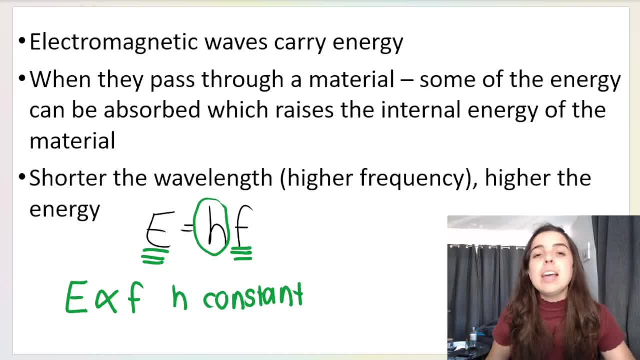 dangerous type of electromagnetic radiation. The other relationship that you need to know is the following, And this we discussed in the previous video C, remember, is the speed of light. It's the speed at which all electromagnetic waves travel, at three times 10 to the eighth. 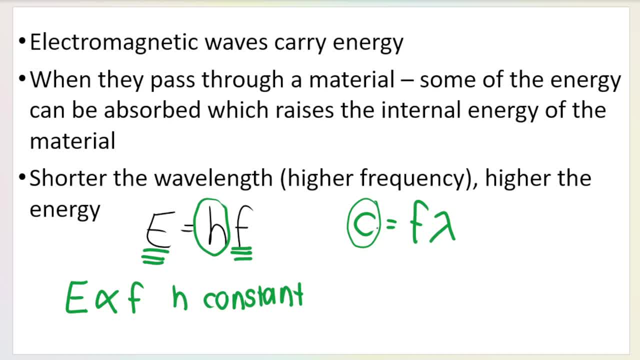 So C is a constant, It does not change. Then, if that is true, which it always is, C is a constant, It does not change. C is three times 10 to the eighth meters per second, and it always will be So, because that is true. we know that. 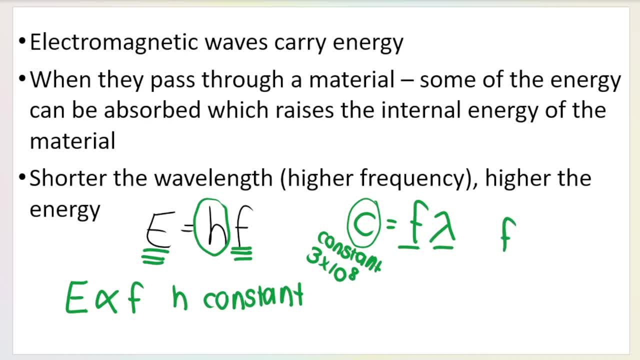 these variables, frequency and wavelength, are inversely proportional, And that's how you write: inversely proportional. So because C is a constant, So what that means great ends is that if my wavelength gets bigger, frequency must get smaller. So if I double wavelength, frequency must halve. If I triple my wavelength, frequency must be a.